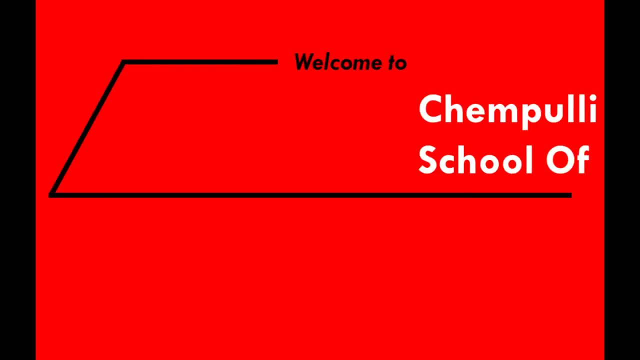 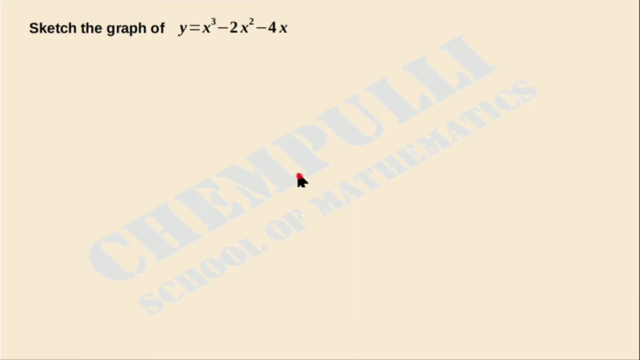 Sketch. the graph of y is equal to x- cube minus 2x, square minus 4x. For that first we can find y intercept. Y intercept means the point common to the given graph and y axis. To find that point we can solve the equation: y is equal to x- cube minus 2x, square minus 4x. and the equation of y. 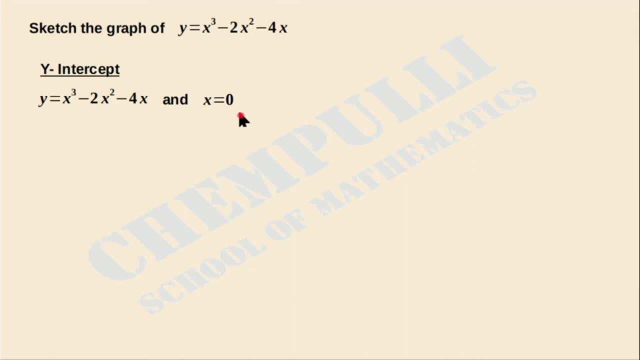 axis, that is, x, is equal to 0. We can solve this equation by substitution method. Substitute this: x is equal to 0 in this equation, Then we will get: y is equal to 0, cube minus 2 times 0, square minus 4 times 0. That means here the place of x we wrote, x is equal to 0. 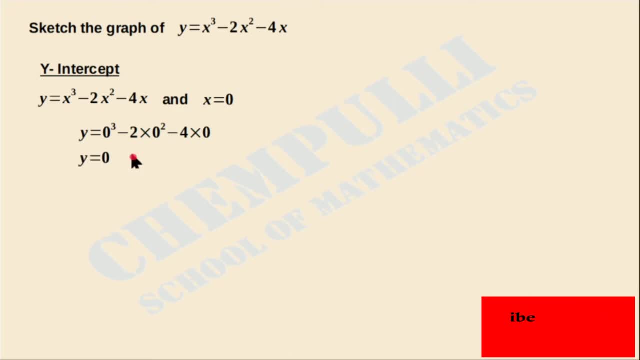 That means we will get: y is equal to 0. That is the y intercept, in this case 0, 0.. That is x value: 0. y value is also 0.. Then next x intercept. To find x intercept, solve the equation: y is equal to x. 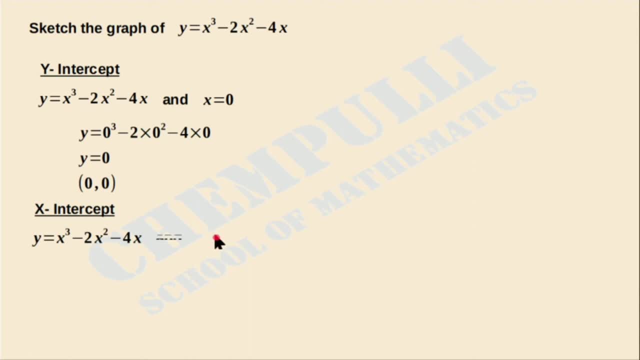 cube minus 2x, square minus 4x and the equation of x axis, that is, y is equal to 0.. Here also we can do the substitution method. Substitute this: y is equal to 0 in this equation. Then the place of y: 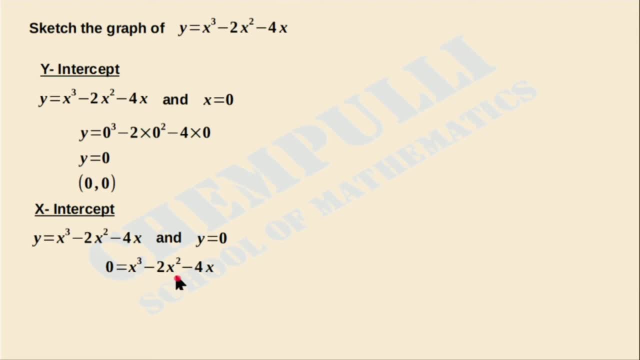 we can write 0.. 0 is equal to x cube minus 2x, square minus 4x. We can rewrite this expression like this: x cube minus 2x, square minus 4x is equal to 0.. Then now you can check this part left. 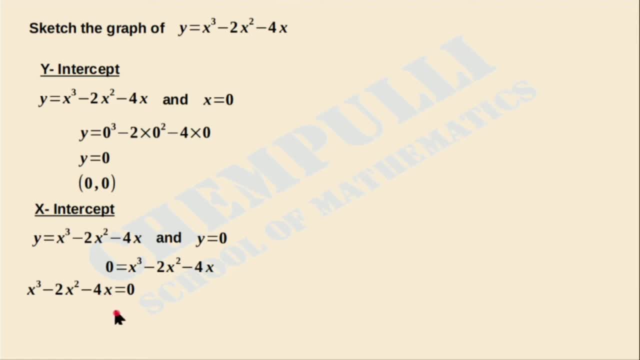 hand side part. Here x is common. Then we can take that x outside. That is x times x. square minus 2x minus 4 is equal to 0.. Now we got: product of two numbers is equal to 0.. That means x is equal to 0. 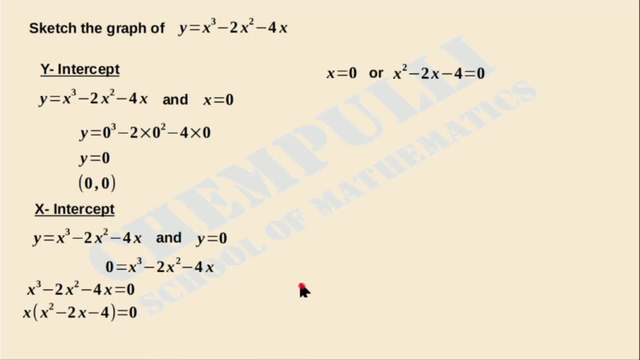 or x square minus 2x minus 4 is equal to 0. Then here, in this case, here we know this, x is equal to 0. Then this case, we can solve this part. Then here first, we can check factorization method. But. 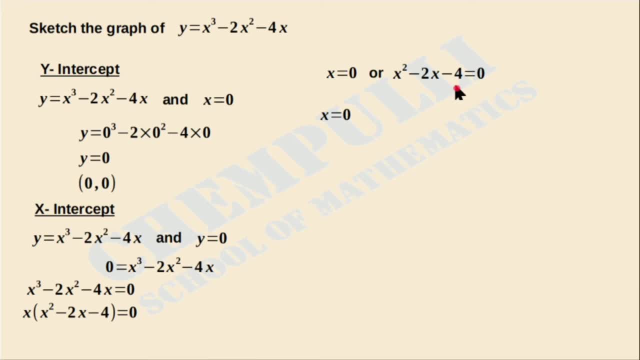 in this case the factorization method is not possible, Then we can solve this part. Then here we can apply formula method. That is, for the formula method x is equal to minus b, plus or minus root of b, square minus 4ac divided by 2a. Then we can substitute values here. x is equal to 0 or 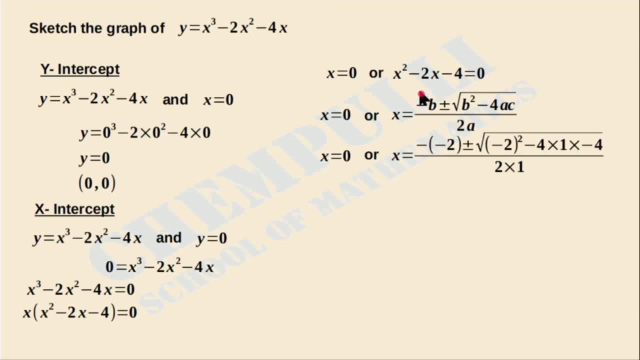 x is equal to minus b. b means the coefficient of x, Then here a means the coefficient of x square and c is the constant number, That is minus 4.. Here, in this case, a is 1 and b is negative 2 and c is negative 4. Then we can substitute that value. 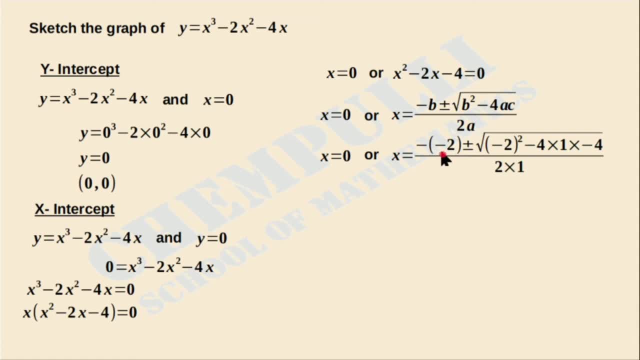 in this part, Then we will get negative. of that is b value is negative 2 plus or minus b. negative 2, whole square minus 4 times. then a value: 1, that is coefficient of x square. that is 1 times. then the c value, negative 4.. Divide by 2 times a, a is, we know, 1, that is 2 times. Then we can substitute. 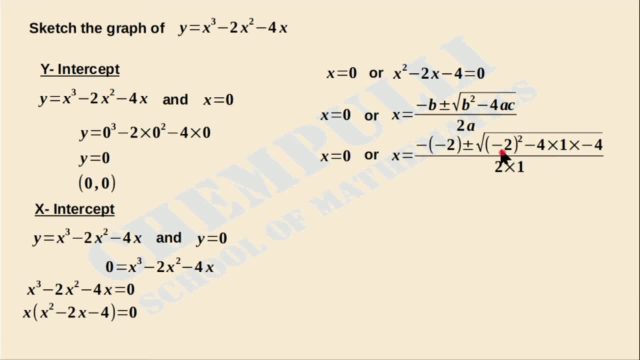 2 times 1.. Then we can simplify this part. First simplify the inside, the root part. Then we can write it like this: x is equal to negative. of negative It become positive. Then next one root of the inside root part, Then it will come 20.. Then 2 times 1, 2. Then that is x is equal to 0, or 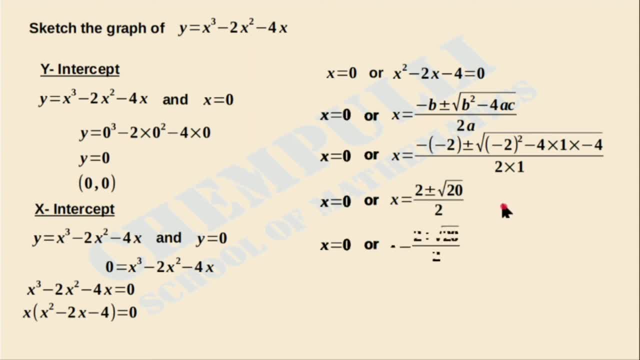 then here: split this one plus or minus. We can write like this: x is equal to 2 plus root 20 divided by 2, or x is equal to 2 minus root 20 divided by 2.. That is, x is equal to 0. or use one. 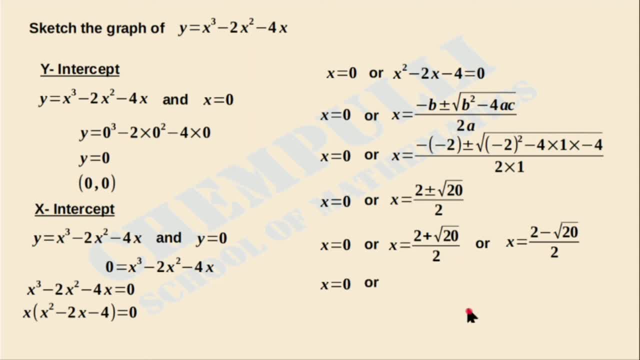 calculator and simplify this part, Then we will get x is equal to 3.24 or x is equal to negative 1.24.. That means we can write this part as a coordinate form. That is x value is 0.. The corresponding y value is 0. That is one coordinate is 0. That is x value is 0. That is x value is. 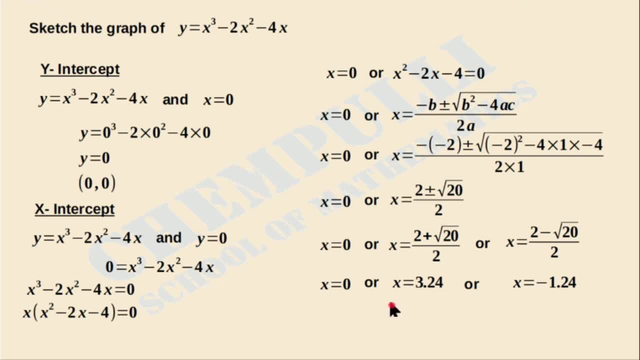 0.. Then another one 3.24.. Then y value is corresponding by 0.. That is 3.24 and 0.. The next negative: 1.24, 0.. That is, we can write that coordinate like this: 0, 0.. Then 3.24, 0 and. 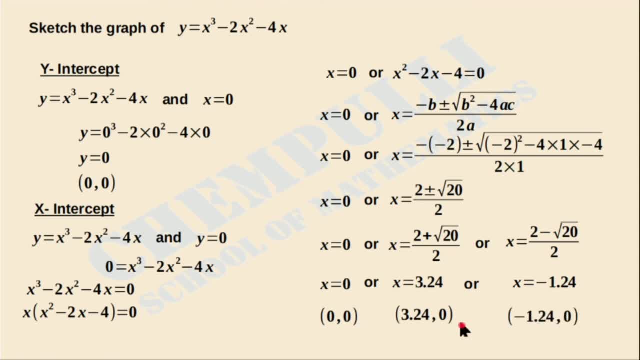 negative: 1.24, 0.. Because in this case all y coordinates are 0.. Because here we know this equation of x axis is y is equal to 0. That is y coordinates, All y coordinates are 0.. These are x coordinates. Then these are the x intercepts. Then next we can find turning points To find: 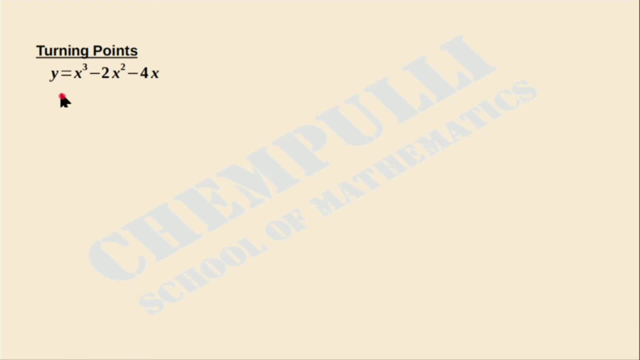 turning points. first we can take the equation of the given curve, That is y is equal to x cube minus 2 x square minus 4 x. Then we can find this turning point, The method of differentiation. Then first we can differentiate this equation That is y is equal to x cube. 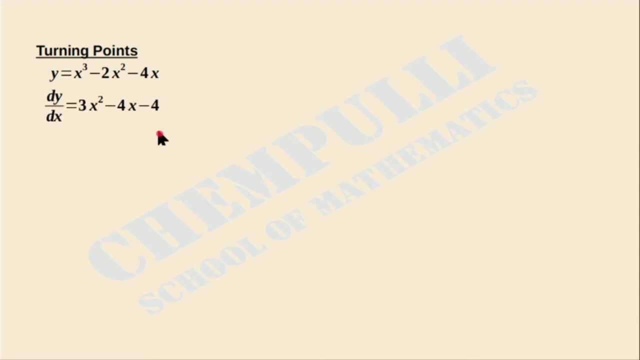 minus 2 x square minus 4 x. That is dy. dy over dx is equal to 3 x square minus 4 x minus 4.. Then to find turning point, first we can take dy over: dx is equal to 0.. That means first we take dy over: dx is equal to 0. That means 3 x square. 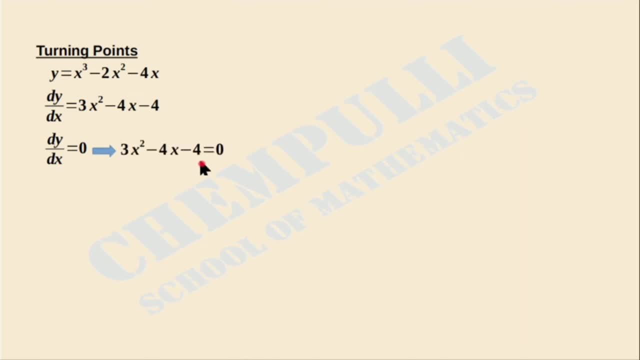 minus 4. x minus 4 is equal to 0.. Okay, Then first we can check the method, factorization method. If factorization method is possible, then apply factorization method. In our case, only apply the which method, That is the formula method. Then first we can check. 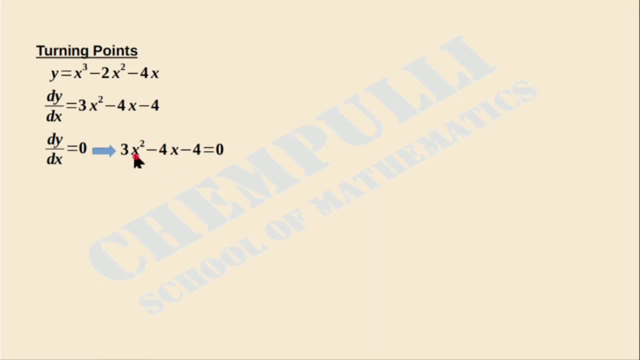 factorization method For that we know here in this coefficient of x square is 3.. Then first we multiply 3 times the number negative 4.. We know 3 times negative 4 is negative 12.. Then we need to find two numbers, The two numbers: product is negative 12 and sum is equal to negative 4.. Then 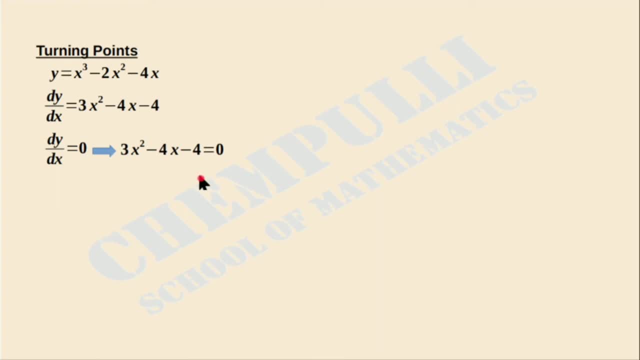 we will get negative. It is possible negative 6 and the number 2. That is negative 6 times 2 is negative 12 and negative 6 plus 2. That is we will get negative 4. That is product of that is we need to find two numbers, That two numbers. product is negative 12. 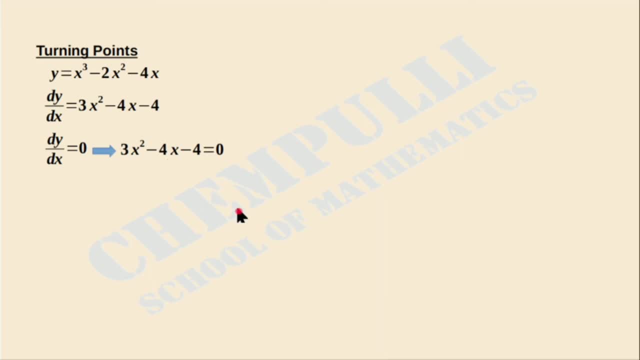 and sum is negative 4. That means we got the two numbers negative, 6 and 2.. Then we can split the middle term by using that two numbers, That is, first write 3 x square, Then the two numbers are negative, 6 and 2. That means we can split this middle term like this: Negative 6 x plus 2 x. Then 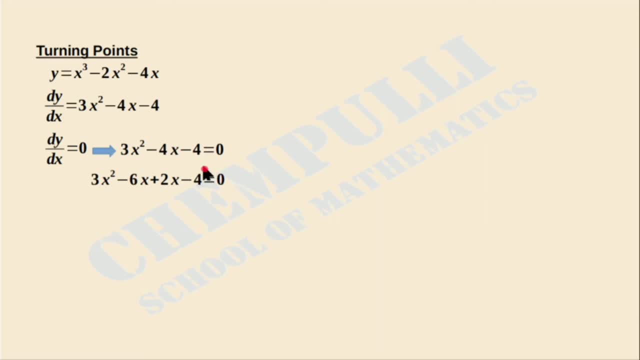 the next number, negative 4, is equal to 0. Here we use factorization method. Okay, Then check the first two times. This first two times case 3 is common. Then also x is also common. Then we can take 3 x outside. Then we will get 3 x times x minus 2.. Then this case 2 is common, Then we can. 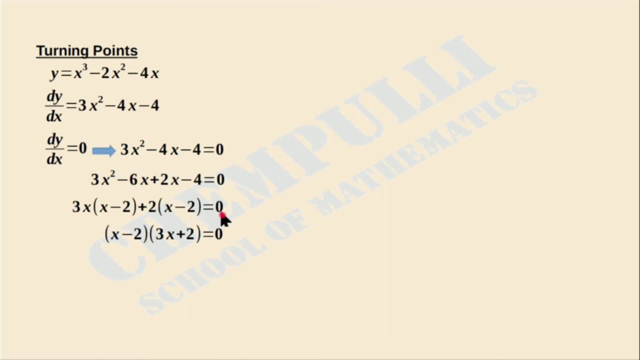 take that 2 outside, Then 2 times x minus 2 is equal to 0.. Now we know these two part x minus 2 is common, Then we can take x minus 2 outside. That is x minus 2 times 3. x plus 2 is equal to 0. 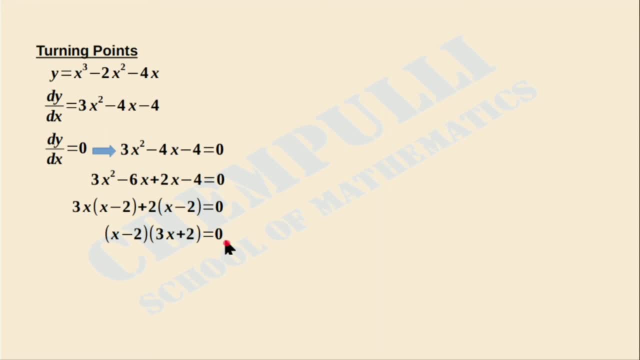 Now we got the product of two term is equal to 0. that means either one term is equal to 0. That is, x minus 2 is equal to 0, or 3x plus 2 is equal to 0. That is, if x minus 2 is equal to 0. It is equals. 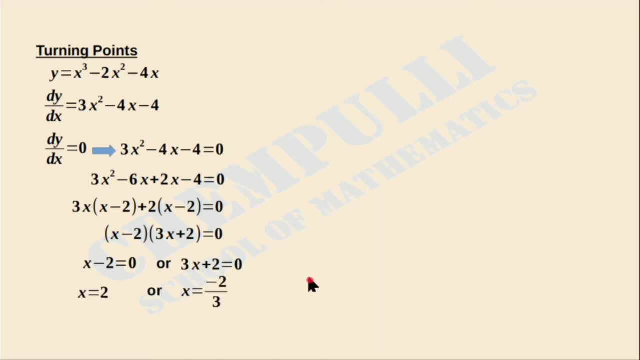 to 2 or x is equal to minus 2, 2 over 3. okay, now we got two value: x is equal to 2 or x is equal to minus 2 over 3. then here we need to represent this value on the graph, then this fraction form. that case is not possible. 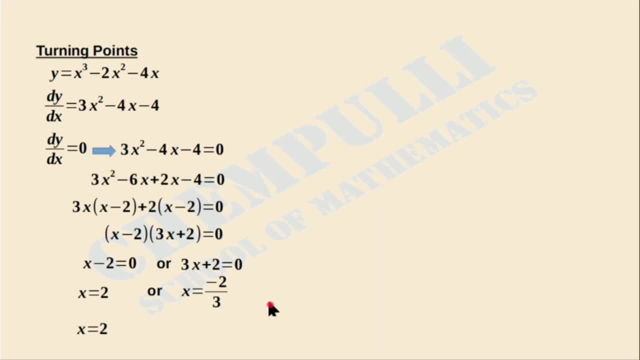 then we can change into decimal form. that means we can write the answer like this: x is equal to negative 0.67. then we can find the corresponding y value. to find the corresponding y value, substitute this value in this given equation. y is equal to x, cube minus 2, x, square minus 4 x. then if we 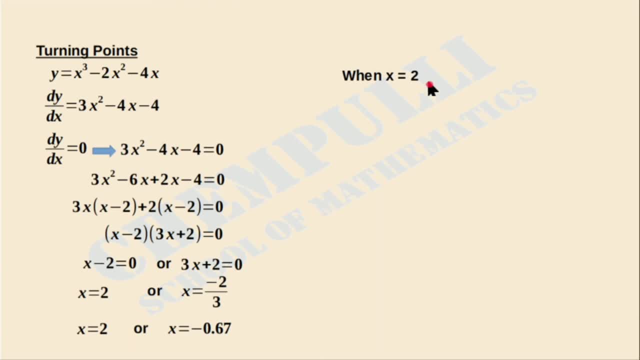 substitute there. first we can take y when x is equal to 2. substitute here: y is equal to x cube minus 2, x square minus 4, x. that the place of x we can write 2. then we will get 2 cube minus 2 times. 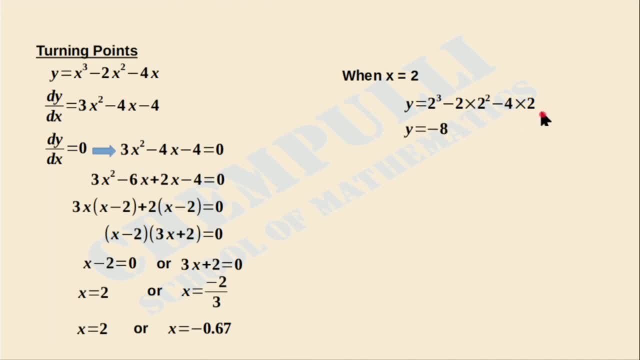 2 square minus 4 times 2, that means we will get the answer. y is equal to negative 8, that is, 1.2 negative 8. to find the other point we can substitute: x is equal to negative 0.67. we know this: negative 0.67 is not. 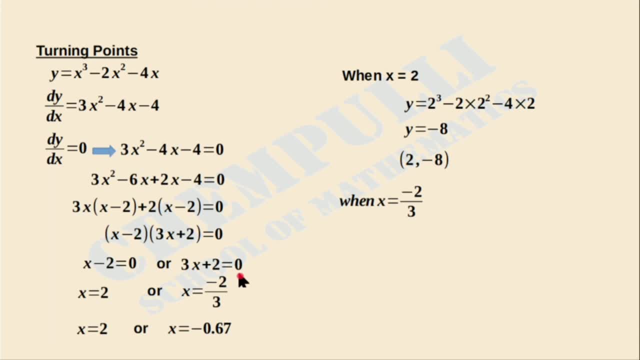 an exact value, then we can. that case we can use which one- negative 2 over 3, then we use here negative 2 over 3, then we can substitute that value in the given equation y is equal to, then if we substitute we will get like this: okay, then we can simplify by using one calculator. we can. 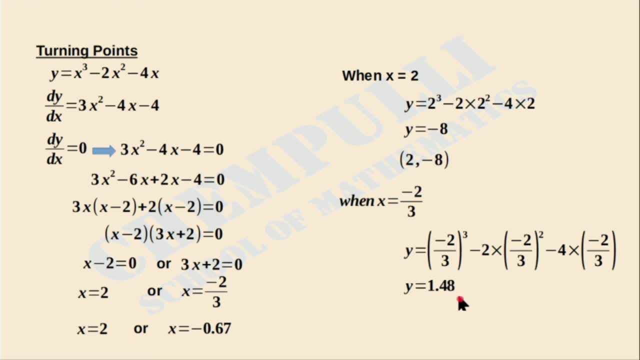 simplify this part, then we will get: y is equal to 1.48. that means the point negative 0.67. we know that in 82 over 3 means say 90, 0.67. then other point: 1.48. that is y 1.48. okay, that is this. 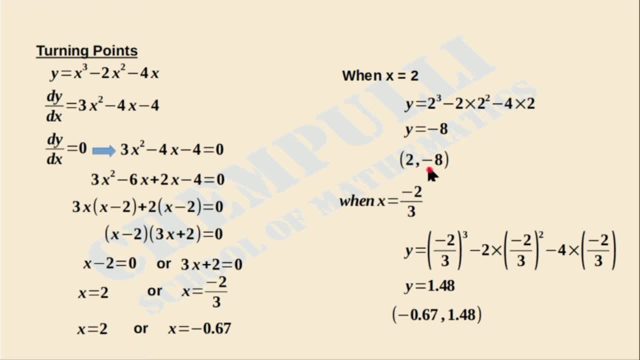 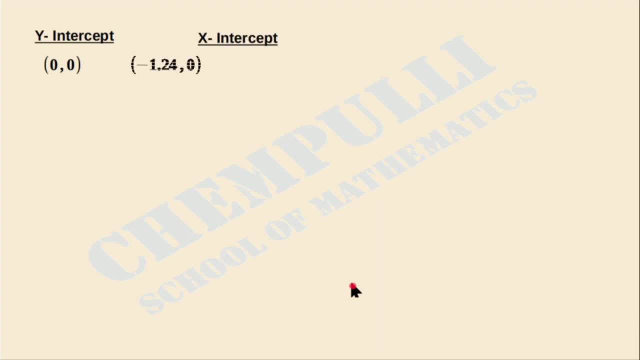 is the one point and this one is the another point. it's the turning point, that is, y intercept, in this case 0, 0 x intercept. there are three x x intercept, in this case negative, 1.24, 0. another one: 0, 0. 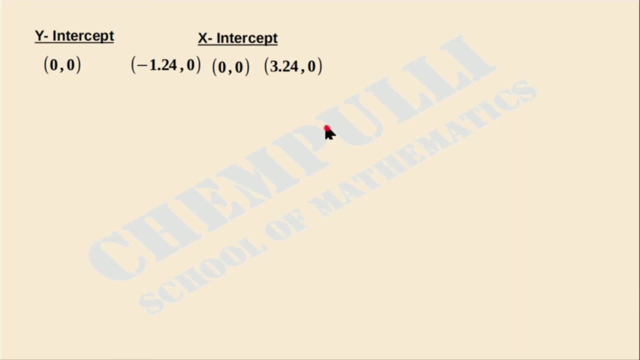 the next one: 3.24, 0. then turning points: 2 negative, 8 negative, 0.67, 1.48. then we can represent this point on the graph. for that first we can take one graph that is x axis is the y axis. then we can mark. 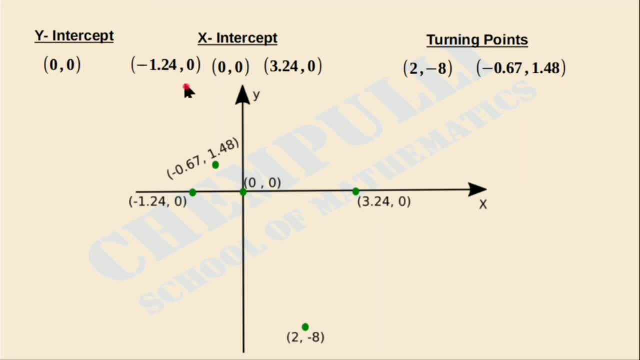 these points on the graph, that is this point, is negative: 1.2 for 0. that is this point. then this point that is negative. 6 point negative 6, 7, 1 point, 4, 8, that is this point. tani point, tani point here. then next 0, 0, that is this point. y intersect and x. 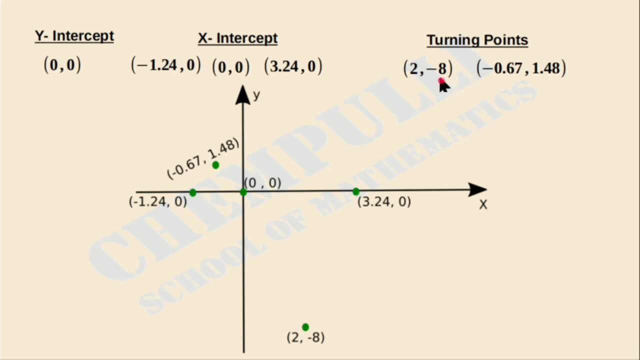 intercept in both case is: the point is 0, 0, then 2 negative 8, that is the tani point, then another one: 3.24, 0, that is this point x intercept. that is this all x, these all values are x intercept then.